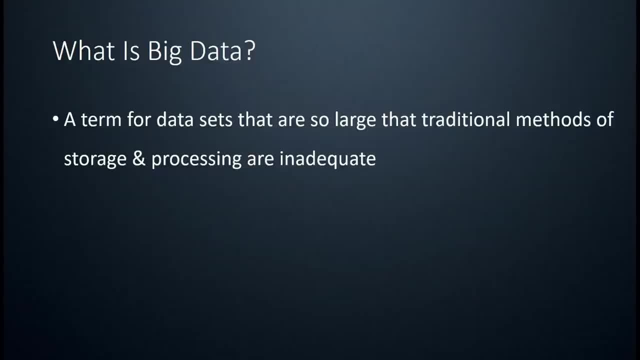 all these different types of data sets. So what this is? they're basically trying to make sure that these databases are working well. with them, It's by means of farming, you know, the cloud, the web, the web apps, all the web pages, the existing websites and all the other other websites that are able to work within those databases. They've become so large that traditional methods of storage and processing are starting to become inadequate. All right, there's been a massive 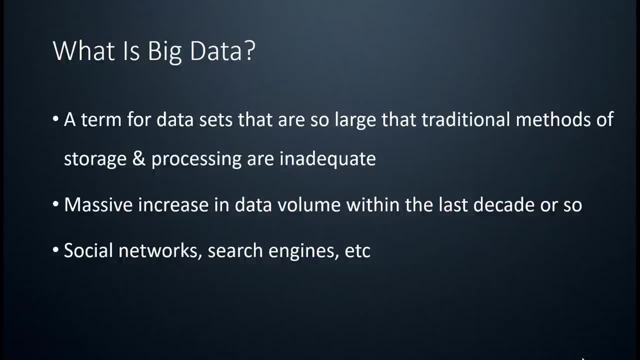 increase in data volume within the last decade or so, and this is mostly due to, you know, huge social networks like Facebook, Twitter, search engines like Google and other websites and applications that store a ton of data. If you think of, you know every Facebook profile, every post in a single day, you can find all these data sets. 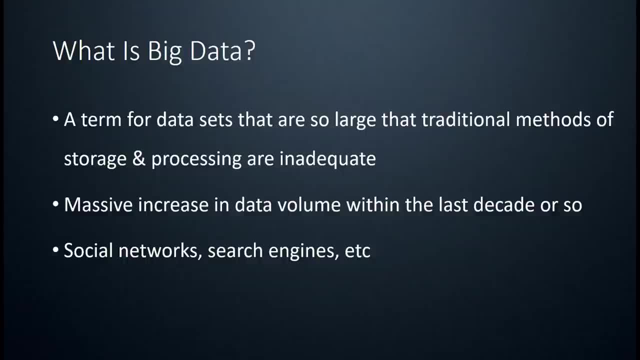 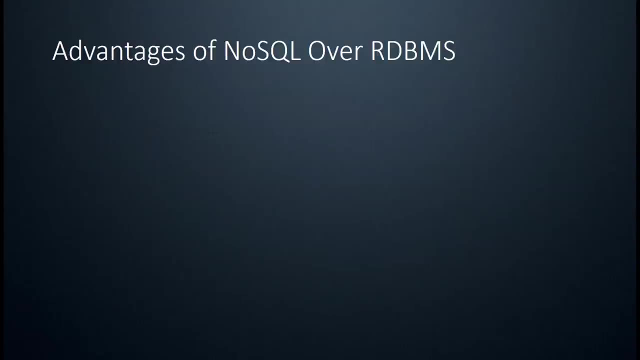 in everyone's feed. that's all stored somewhere and that's just a huge amount of data, and some of the challenges with this, with this data, is storing it, capturing it, analyzing it and transferring it- all right, so so this is where no sql comes in now, please don't think that anything. 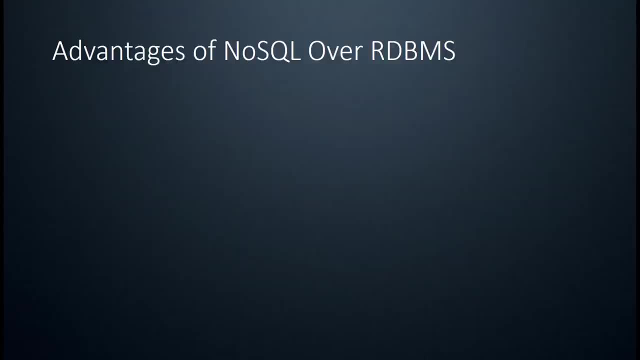 that i say in this video is: uh, you know, please don't think i'm saying relational databases are dead. no sql is going to take over the entire industry. anyone that says that has absolutely no clue what they're talking about, or they're just trying to sell you something, some kind of no sql. 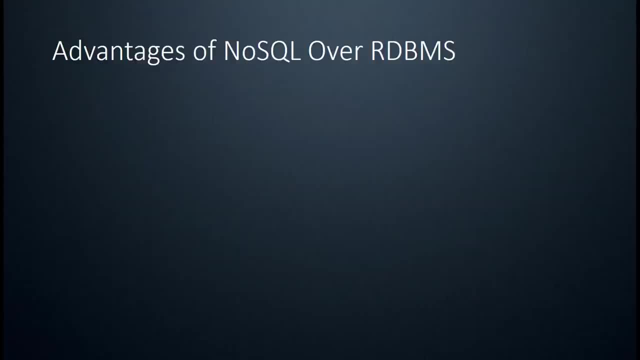 service. there's a lot of situations and a lot of applications where a relational database is the obvious tool. no, sql and relational databases, kind of like a hammer and an axe. they're both going to be useful. they're always going to be useful. they just have, you know, certain purposes. you're not. 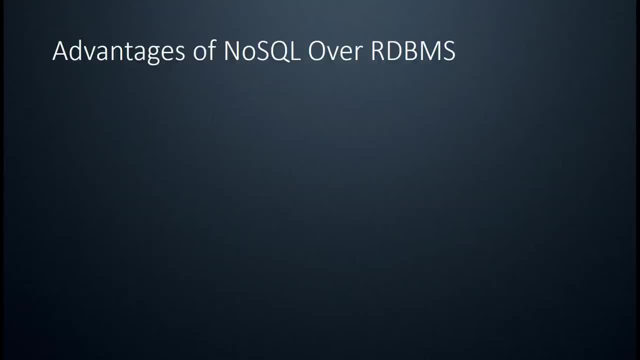 going to use an axe to to bang in a nail. you're not going to use a hammer to chop down a tree, but they're both necessary, all right, and we're also going to talk about the advantages of relational databases. so we've already discussed big data and how you know it's a huge benefit of. 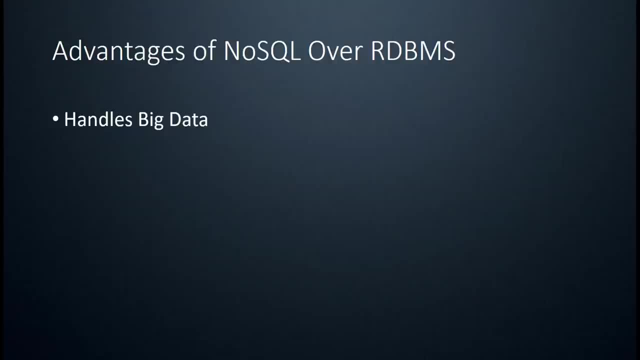 no sql is that it handles a lot of data and it does it very quickly. another huge advantage is data. it's data model, which is extremely flexible, all right. so if we look at relational databases like, let's say, mysql, sql or postgres, we have to go in and structure the data in a predefined schema. you guys that. 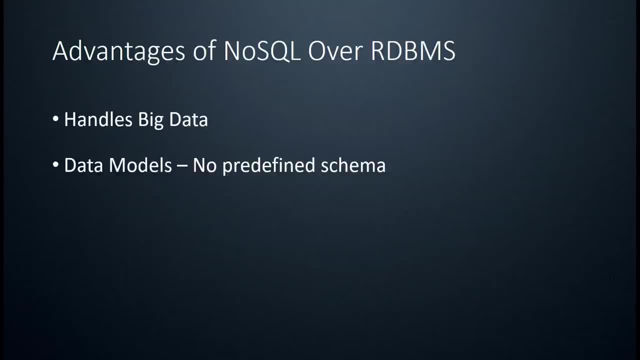 have worked with sql know that you have to go in and create the database. you have to model everything that you need: the tables, the, the fields, the constraints, even the data type of each field. all right, so is it a varchar? is it text and integer, and so on? and this is all stuff that 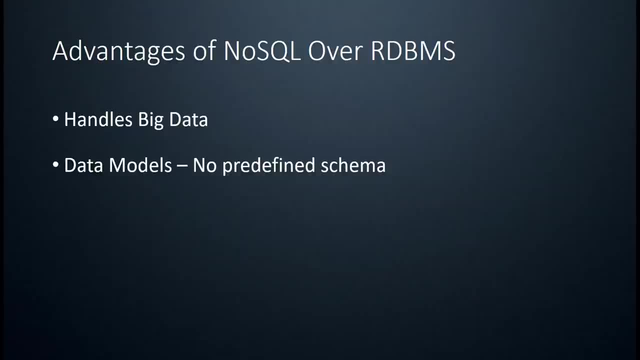 you have to do when you're working with relational databases. yes, you can find tools that can make it a little easier, but at its core, at its core level, this has to be done in the data layer. this brings us to the next advantage, which is the data structure. not only do you not have to define, 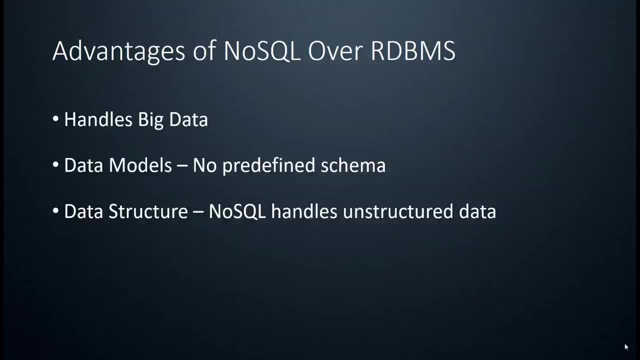 your tables and columns. well, there is no tables and columns, but you don't have to define anything like that. you don't even have to know your data structure now, unless it's going to be a completely dynamic data model. you should at least plan out and have an idea of how your data is going to look. 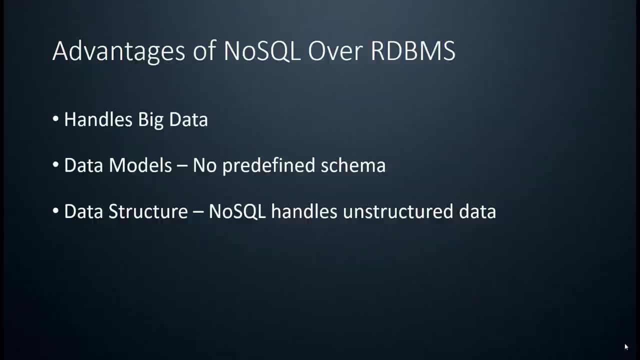 and how it's going to look in the application layer. okay, there's a lot of different tools. there's object relational mappers that we can use to actually create a schema on the application layer. all right, so hopefully that makes sense. no, sql databases are in many cases much cheaper. 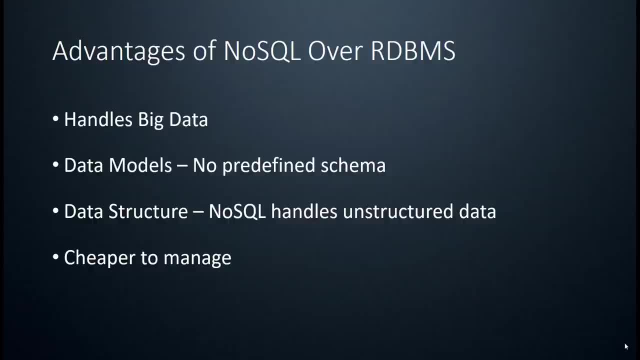 than to manage, than relational databases there is, you know, there's less of a need for multiple system admins because there's not. there's not as much to do, okay, there's not as much to manage, so that's going to be cheaper. so let's talk a little bit about scaling and what scaling is a huge advantage of no sql it uses. 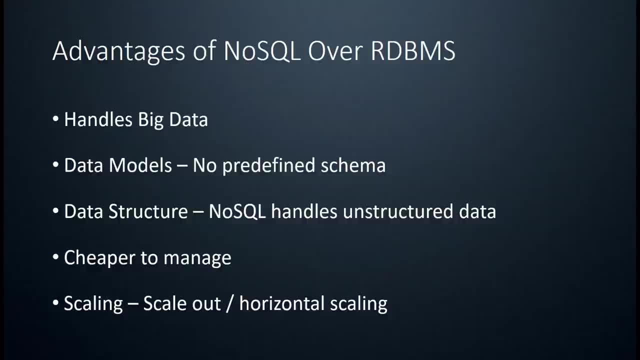 something called horizontal scaling or scaling out, versus a relational database which uses vertical scaling or scaling up, and i'm going to go over what this means in a second. but scaling is is extremely important in this industry because it's always growing. successful websites and applications are always going to gain more users and more data. facebook is never going to really. 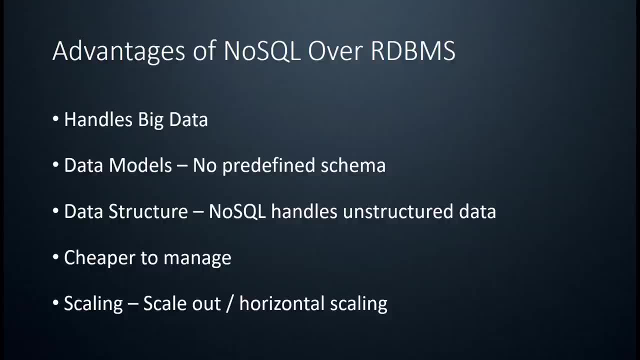 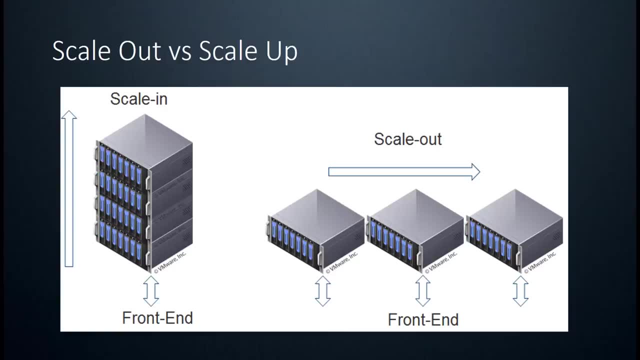 unless they they get rid of critical parts of their interface and their functionality. so scaling is definitely key when you're working with lots of data. all right, so let's take a look at an image here that kind of shows you scaling up versus scaling out. all right, now this image on 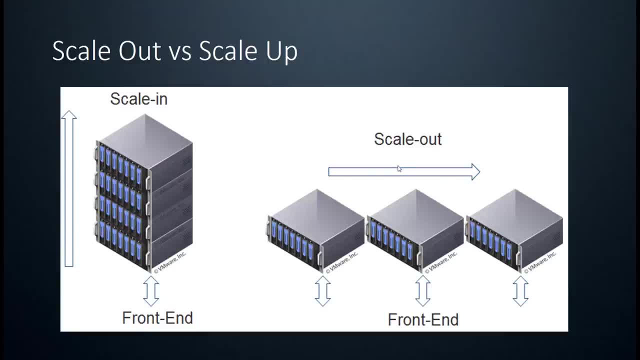 the right here. scaling out is also known as horizontal scaling, and this is what no sql databases do. and then over here is an example of scaling up or vertical scaling, and i know it's a scale in, but this image is close enough to explain what i'm talking about. so let's start with scaling. 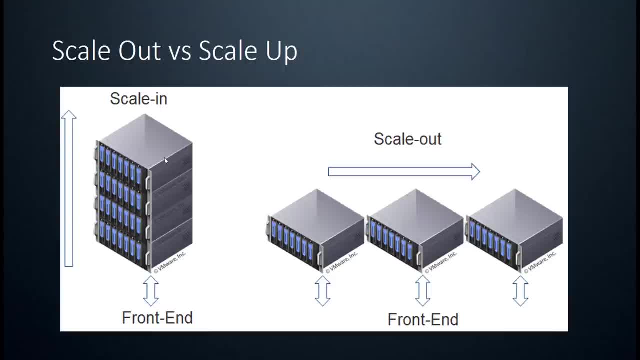 up, okay, which is relational databases. so this means that in order to scale and- uh, you know, build up our system, we need to add components, so we need to add storage, you know, drives, memory, cpu, power, network ports and other resources that are very, very expensive. so it's easy. 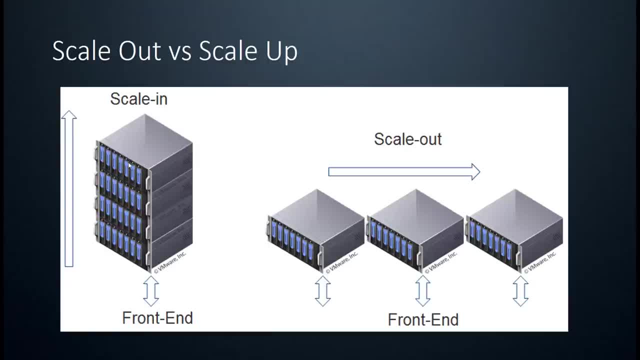 to see that that there are some hard limits just by looking at this, because obviously you can only put so much into this one box. you can replace it with a bigger box and a bigger system, but you're talking about huge amounts of money and huge amounts of time. 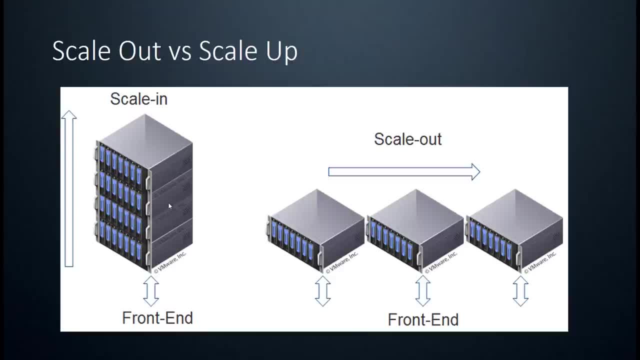 so the huge downside to this method is limitation and cost. now scaling out, or scaling horizontally, which is what most no sql systems do. this means that you can use much cheaper commodity hardware and you can simply add additional nodes, expanding your disk size, your your memory and so on. all right, and a group of nodes like this is called a cluster, which you 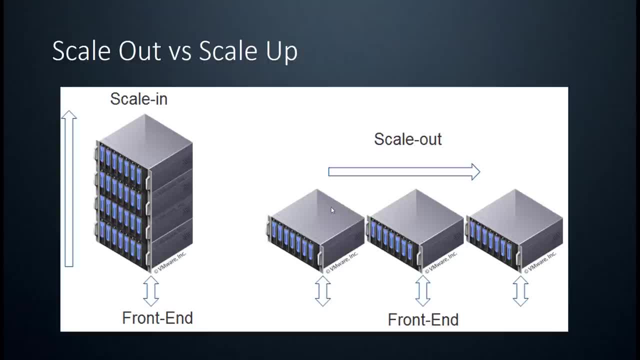 may have heard before, once you reach the limitations of of your cluster, of your nodes, you can simply add another one, and for a fraction of the cost of of. you know, if you were scaling up and you were adding these expensive components, uh, or even worse, if you you were to the max and 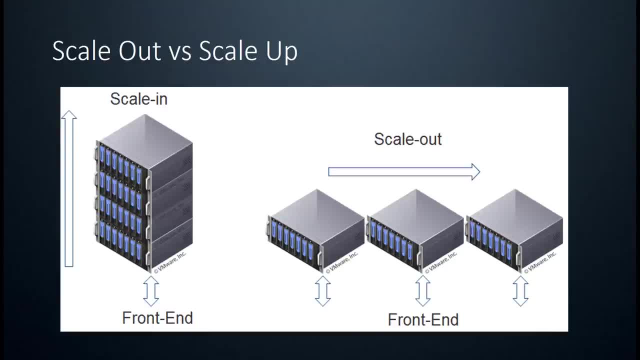 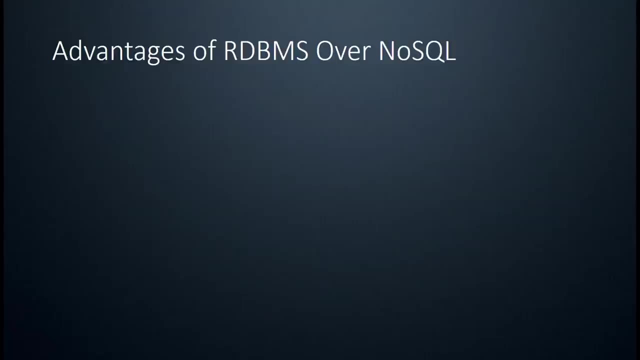 you needed to still scale up, you'd have to. uh, you know you need a whole new infrastructure, which can be a huge pain in the ass. so no sql. you know scaling is definitely one of the advantages. all right, so now let's talk about relational databases and what they have over. no sql databases. 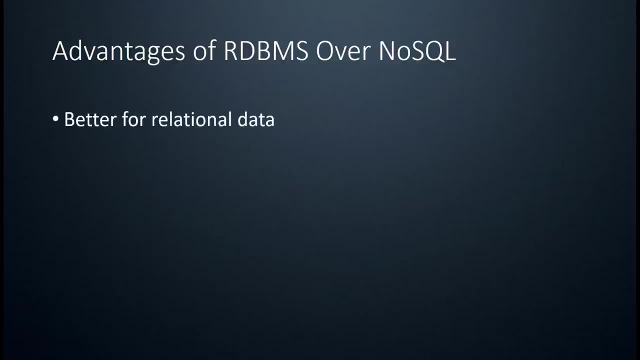 so you don't have to know much about any of this to guess that relational databases are great for relational data. you have a set of relational databases that are great for relational data schema, where you always know what columns exist for a certain row. you know that a user can have a 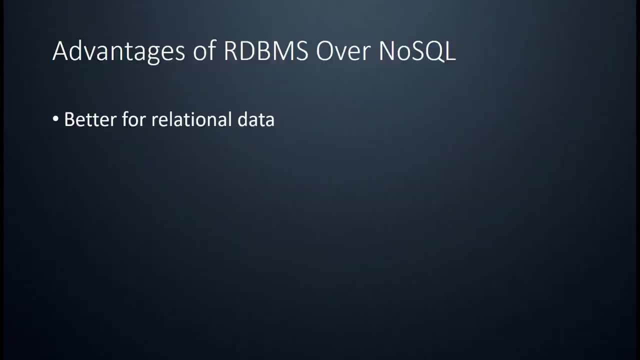 blog post. you know exactly how these two tables are related. even though being schemaless is looked at as a plus in many cases, having a set schema also allows you to better understand the structure and the relation of the data stored. all right, it takes more maintenance, and so on, but 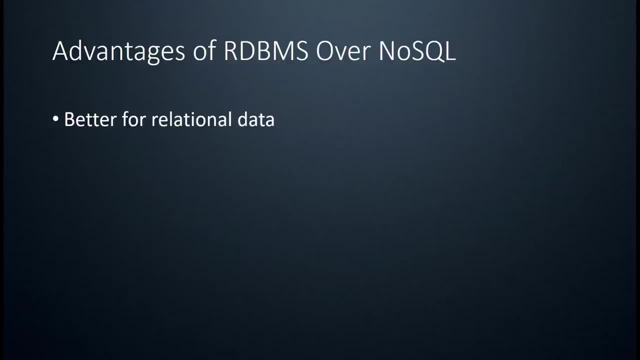 it is safer. in many cases where data is closely related, this type of database is a actually the better choice. okay, relational databases also use something called normalization, which organizes data in a way that eliminates redundancy, so all the data is stored in one place. normalization is really important because it allows a database to take up as little space. 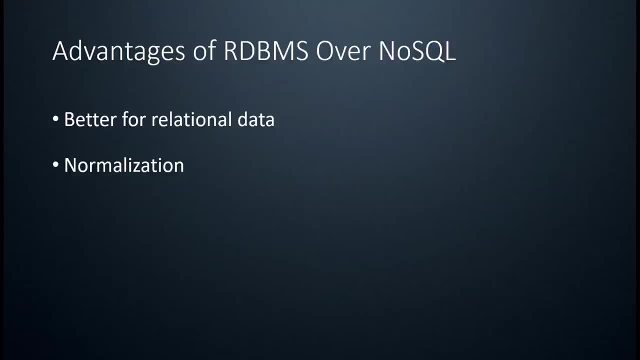 as possible, which also results in better performance. now there's all types of normalization. there's one, nf2nf, and it gets really complicated. i'm not going to get into that, though that's a whole. another video on its own relational databases also use sql or structured query. 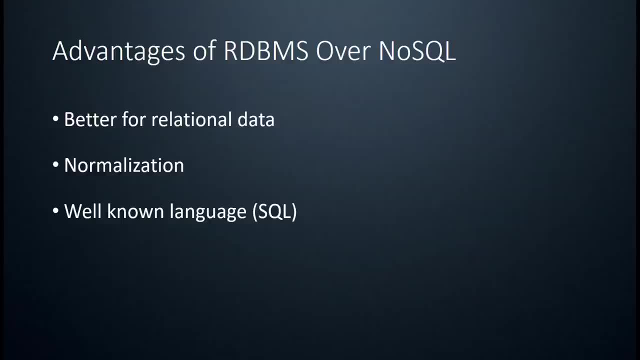 language, which is an old technology but very solid and in, in my opinion, very easy to learn. most sql or relational databases also allow you to enforce data integrity rules using foreign constraints. so to give you an example, let's say that we had an author's table and a blog post table and we had a data integrity table where figur Sheikh Jamal had a blog posts table and we had an authors table and a blog posts table. Davert's table as well kept on the most data integrity using foreign constraints. so to give you an example, let's say that we had an author's table and a blog posts table and we had a school today and the social data integrity table is based on string philosop, trem point and an authorization table in a language department and, according to lockerESS, different. 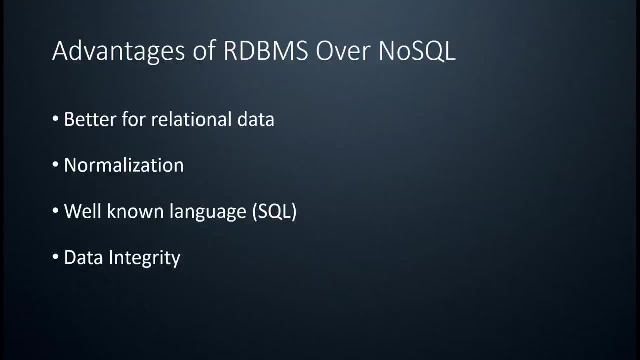 an author that created a post. well, we can create a constraint so that we wouldn't be able to delete a user that had written a post, because if we did that, we would have a post with no author, okay, or no user. we don't really have these constraints available at the data level in no SQL. so the last advantage: 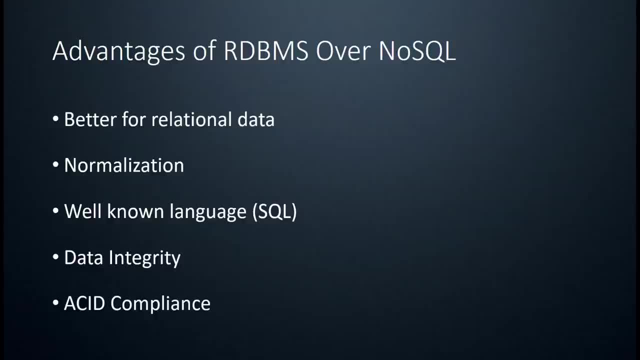 here is that a lot of relational databases are acid compliant. so this is- it's an acronym- it stands for atomicity, consistency, isolation and durability, and this is a kind of a complex topic so I'm not going to go into depth. but the gist of it is that it's an all-or-nothing rule. so when we make database, 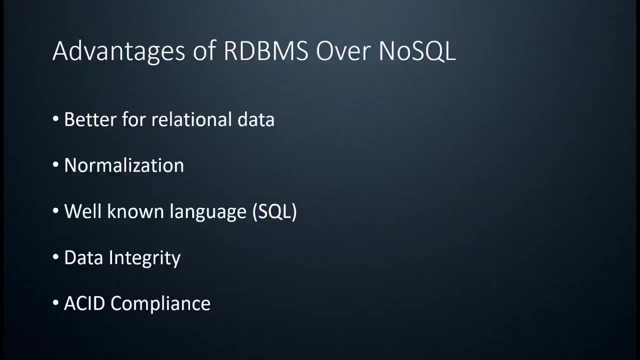 transactions, for example of a bank account transfer, let's say, from one account to the other. we have a series of actions for that. so we have to do multiple queries, we have to take money out of one account and then we have to put it into a not-for-profit. 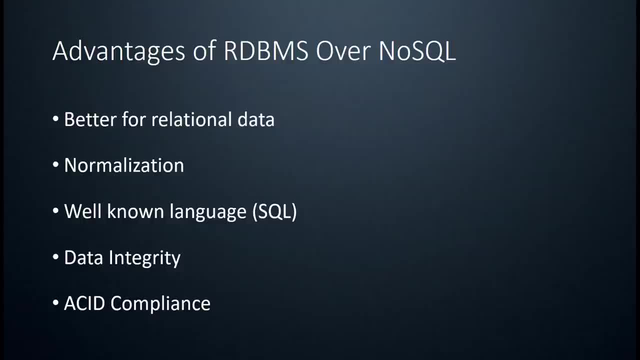 we have to do some math and tallying and so on. well, most relational databases can use acid compliance to say we're either going to do all of all of the actions or none of them. because could you imagine transferring money to you know, from one account to another and only the money gets taken out from the first account? 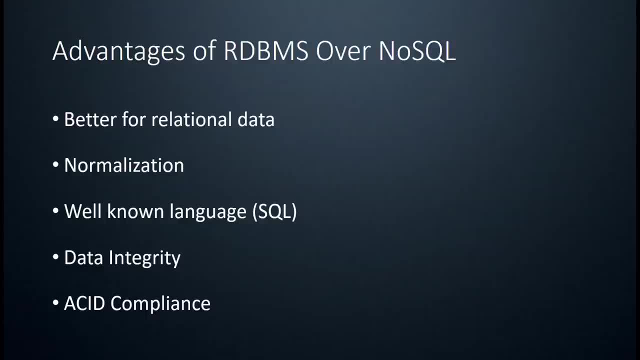 and then something goes wrong, it crashes and it never goes into the other account, so that would cause mass havoc. so this is something that's very important. and now, this isn't to say that we can't do that with no SQL, because we can. it's just not built into the core system at the level that relational it is with. 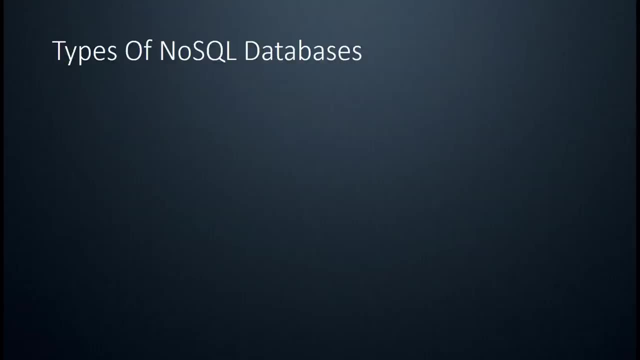 relational databases- alright, so hopefully that makes sense now. now that we looked at the advantages and disadvantages of both relational and no SQL, let's talk about the different types of no SQL databases. alright, now, there's actually more than this, but these are by far the most common. 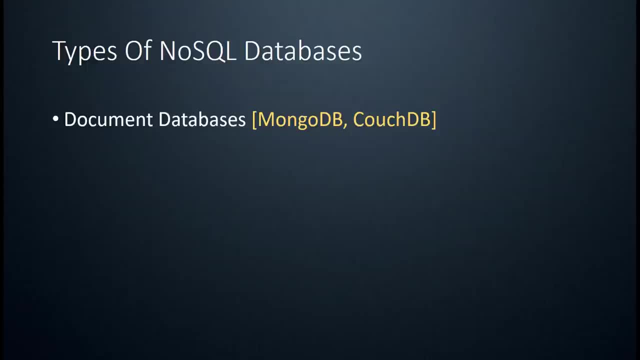 you can see that there are a lot of different types of relational databases. so first we have document databases and the most popular document database- or no SQL database in general, is MongoDB. I have a crash course on MongoDB which I would strongly recommend watching after this video if you haven't already. 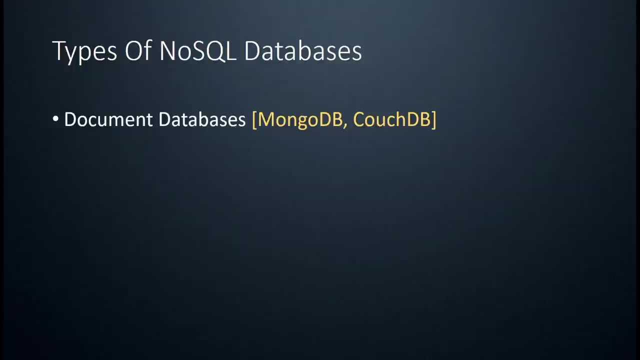 document databases store data similar to JSON or JavaScript object notation, where we have curly braces inside that we have key value pairs. they can hold strings, numbers, arrays, images and so on and so forth, embedded objects and so on. now, on the database level, they're completely schemaless, so your application can be very dynamic. if you wanted to have, let's. 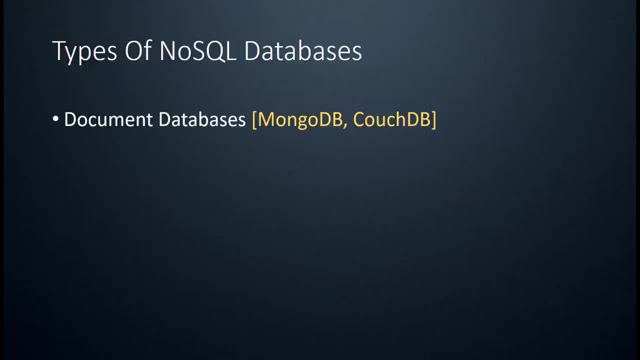 say, users be able to add custom fields to their profile. a document database is definitely the way to go. one profile may have an address, one may not. some may have BIOS or contact info, some not. so with relational databases we would have to, we'd have to strictly define everything from. 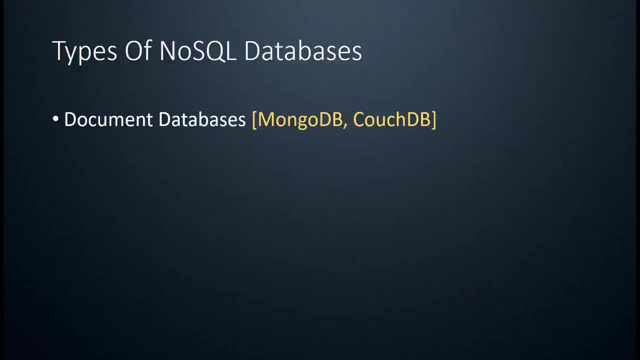 the table to the fields and so on. so this would not be ideal for something like that with dynamic data. so we also have column databases, which is optimized for reading and writing data in columns instead of rows. an example of this would be Apache Cassandra. this is a great. this is great for things like analytics and 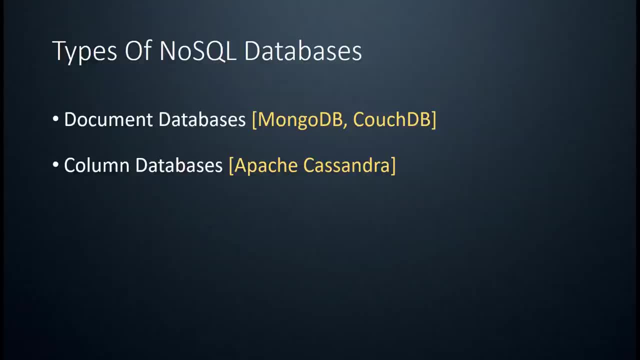 it reduces the overall disk i o requirements and the amount of data that needs to be loaded from the disk, So it can be quite optimized. Then we have key value stores, which is the simplest type of NoSQL database. You have a key and a value. 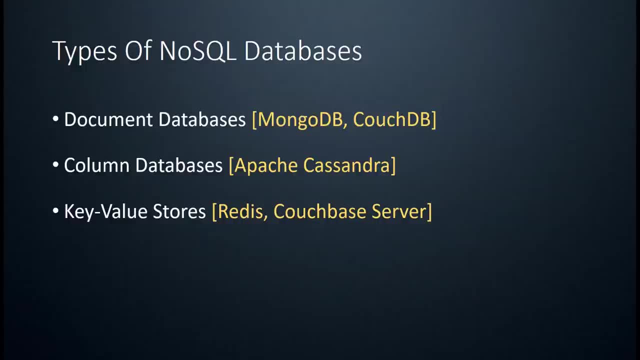 This is optimal for huge data sets with very simple data. It's extremely fast but not very intricate and customizable, And it's similar to an associative array or a hash. Now we also have cache systems like Redis, which is also a key value store. 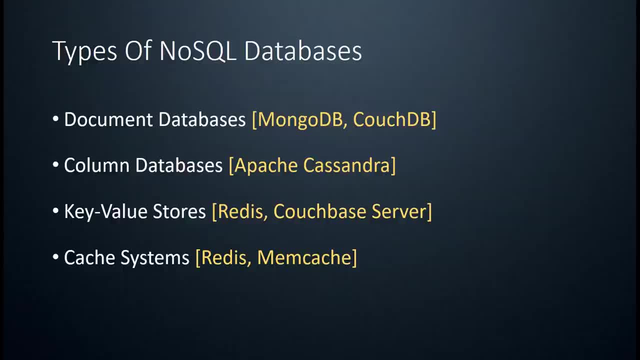 but can also be used as a cache system for temporary values. Redis can be used as a database and actually write data to the disk, or can just store data in cache. All right, I have a crash course on Redis on my channel if you want to learn more about that. 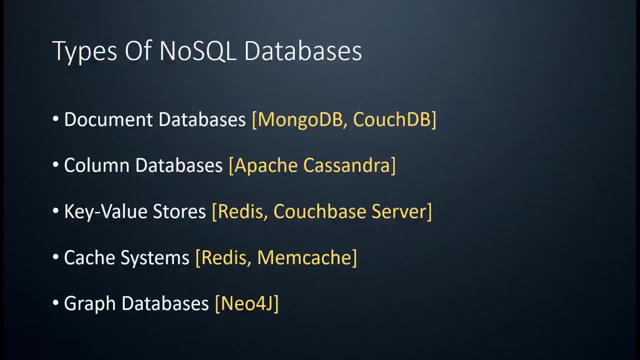 So next we have graph databases, which aren't that common, but I think they're very interesting. I actually did a course on Neo4j, which is the most popular type of database. Everything in a graph database is looked at as a node. 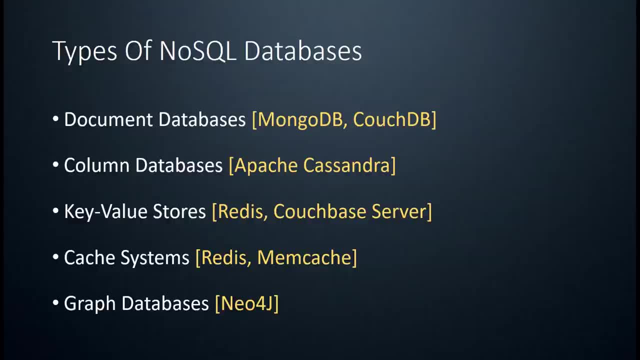 and they can have relationships with other nodes through what's called an edge. All right, so if you have some extra time, I would definitely suggest checking it out. looking at Neo4j, because it's really interesting. These are used for huge data sets, like social networks, where everything is related. 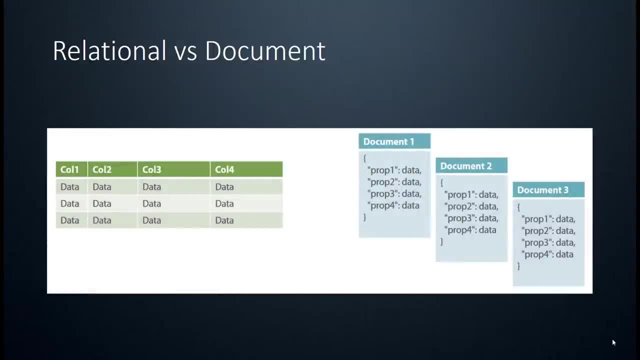 All right. so before we go, I just want to give you a visualization of a relational database, on the left, with columns and rows, And then on the right, we have a document database which has a very similar structure to JSON. All right, now the relational database. these all have to be set.